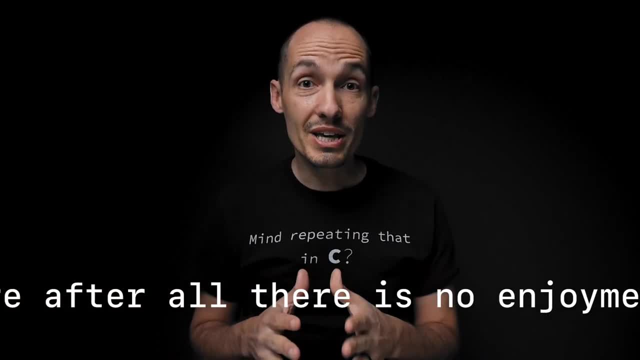 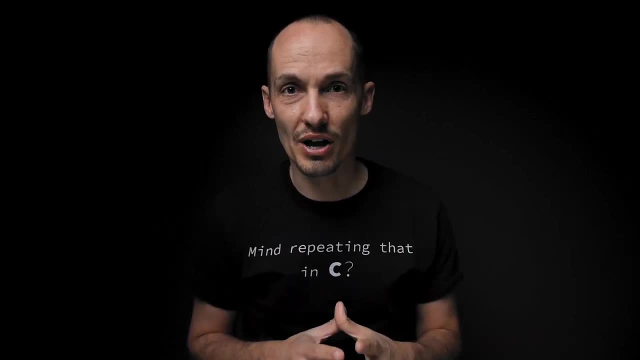 talk about strings. we could be talking about strings of characters, but we can also be talking about any sequence of symbols. So any sequence of symbols can do the trick here and we'll work with a try. This could be strings of binary bits, but it could also be ASCII characters, which is 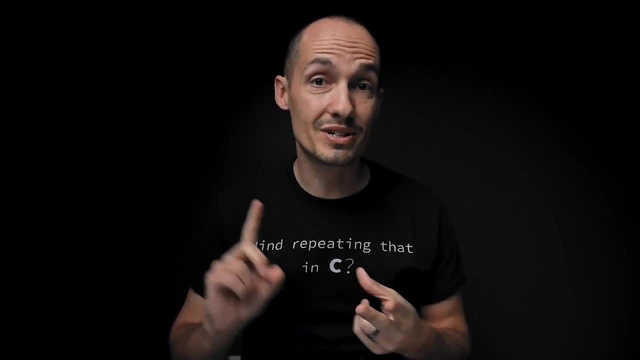 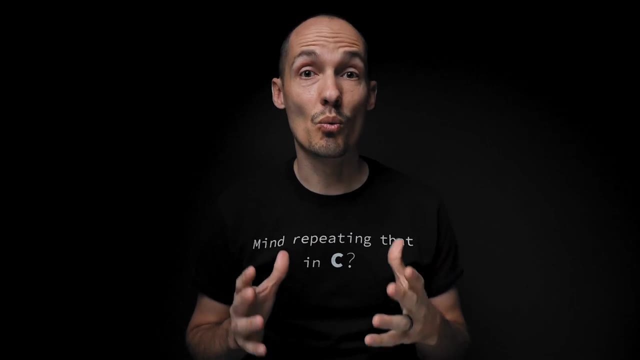 what we're going to use today. So tries are also sometimes called prefix trees or digital trees. So if you hear those terms, we're talking about the same thing. So the main thing is: a try is going to allow us to efficiently check whether or not a particular string is in. 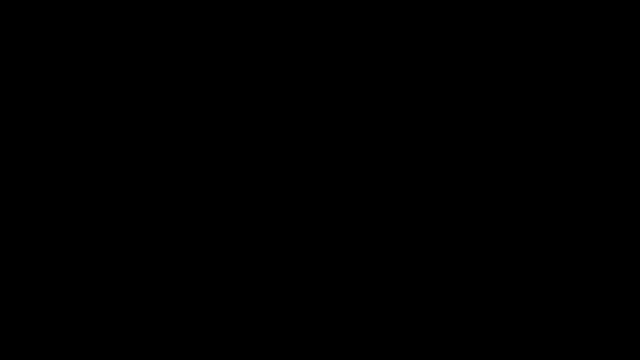 our set of strings. So let's look conceptually at how this works. Like I said before, a try is a tree, So it has nodes, and each node is going to represent one symbol in a sequence And the node's children are going to represent all of the symbols that could come after that symbol. 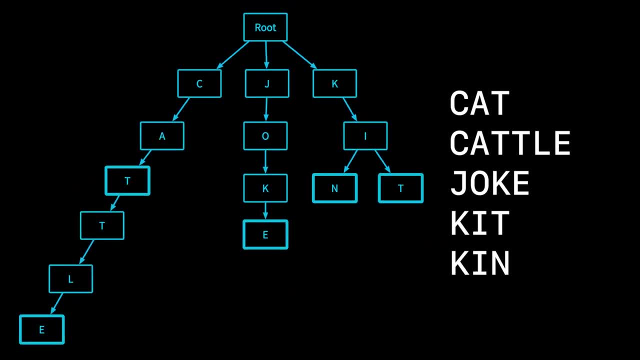 So let's say I want to store these strings in a try. So if I store these strings in a try, it would look something like this: You notice that each node represents one symbol and we can move down the tree to see if each word is contained in it. Also, notice that 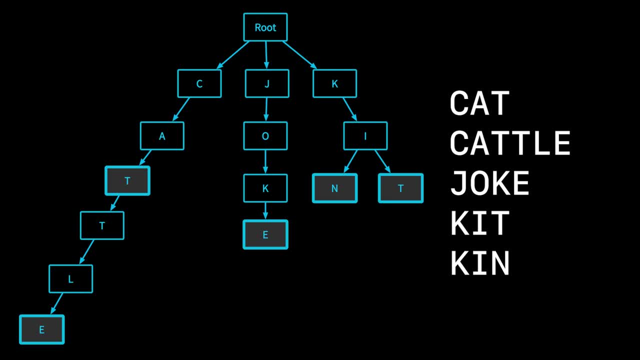 I have bolded the terminal nodes, That is, the nodes that represent the end of a string. So we have to mark those nodes or we wouldn't know whether or not say cat C-A-T-T with two Ts isn't also one of our words. Now, sometimes you will also see tries shown like this with: 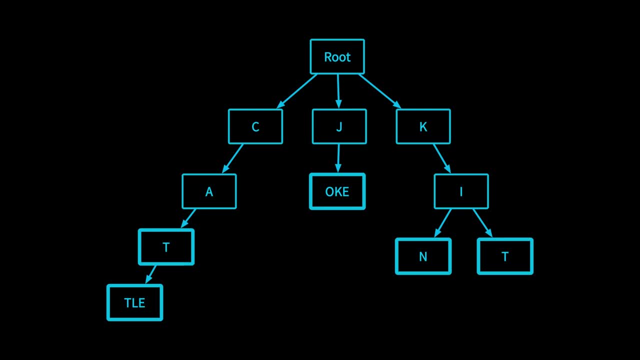 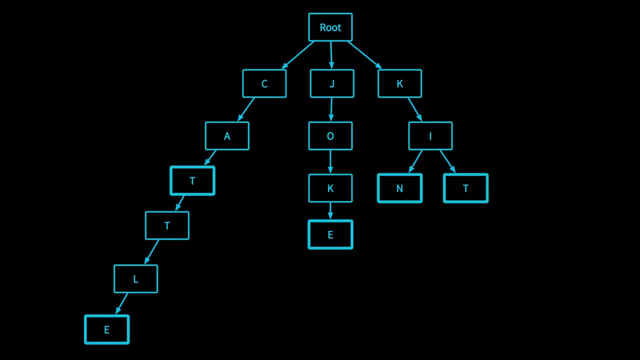 one node representing a substring. This representation naturally produces smaller trees with fewer nodes, but it also is a little more complicated, And so, for simplicity, today we're going to stick with one symbol per node. I'll leave the substring nodes as an exercise for you or maybe a topic for a future video. But so why is this a good? 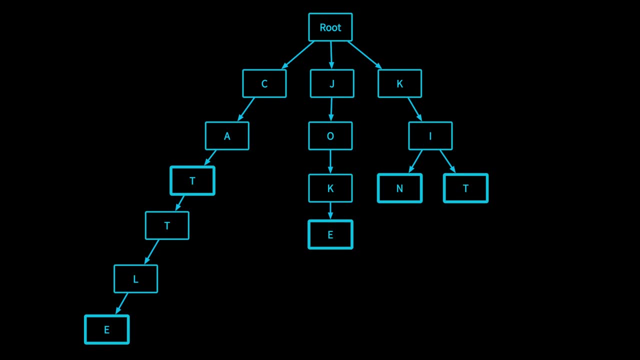 way to store a set of strings. Well, the main reason is that some key operations- inserting new strings, for example, deleting strings and, most importantly, searching to see if a string is in the set- are quite fast And they also scale well. So look at an example. 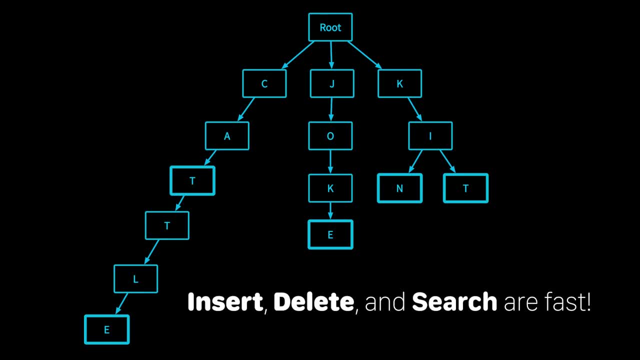 Say that Let's see if cat is in the try. Well, I start at the root and I can see that C is one of its children, so that's great. And I can see that A is one of C's children and T is one. 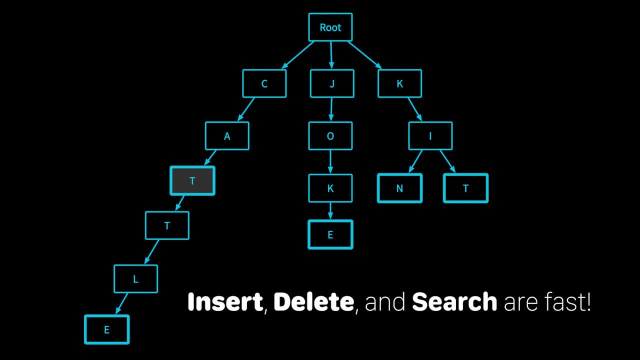 of A's children. And this T node is marked as terminal. so I know that cat is stored in my try And that operation is going to stay the same, regardless of how many other strings I store in this try. I mean, I could store 10,000 strings in this try and it would. 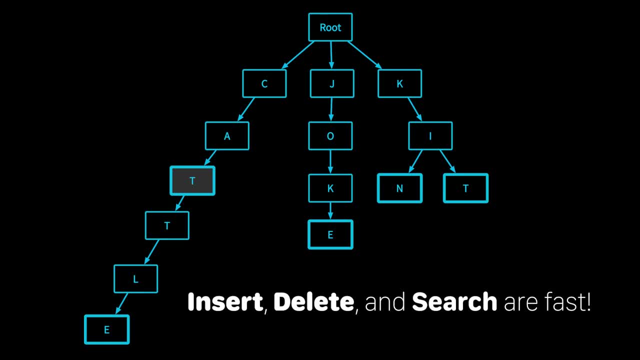 take more memory to store, of course, but finding cat in this try would not change. It would take the same number of strings. So that's really nice, And that's also true when we insert stuff and delete stuff to and from our try. 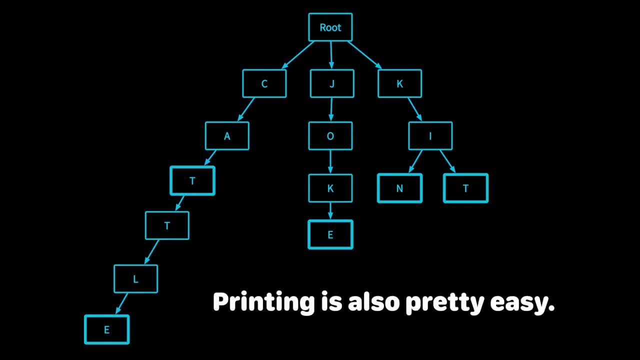 Now, another nice feature of a try is that it's also very straightforward to print out strings in the try in sorted order, and that's basically just using a simple depth first search. So we'll talk more about that later, But this makes the try a solid data structure. 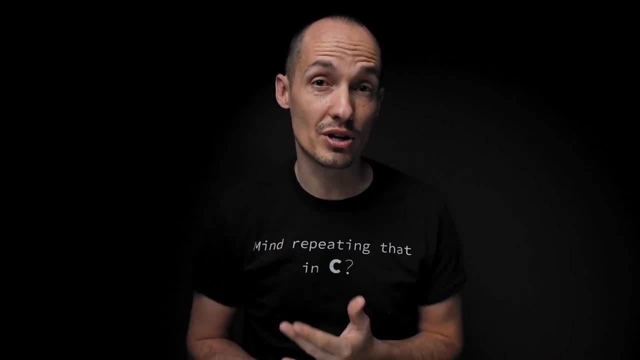 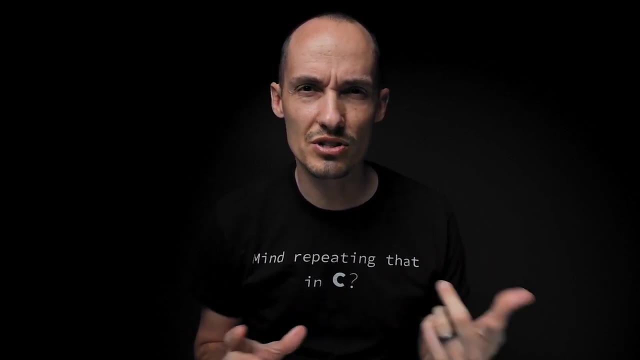 for people who want to store sets of sorted searchable symbolic strings. Wow, try to say that fast. Sets of symbolic searchable sorted strings, certain sorted strings of of searchable sorted sets of strings, Anyway, lots of S's. That's definitely trouble. 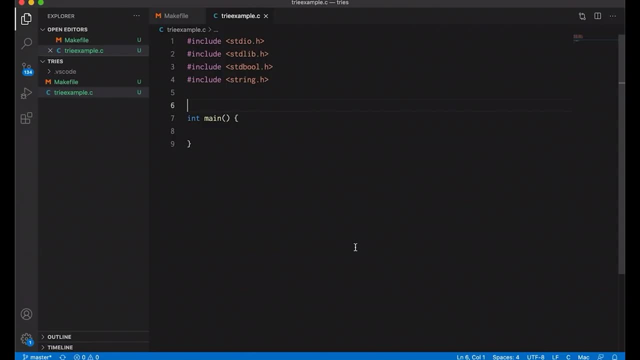 but enough about the conceptual stuff, Let's get into the code and see if we can build one of these. So I'm gonna implement this try in C, though it would be fairly straightforward to report this to C++, Java, Python, Ruby. 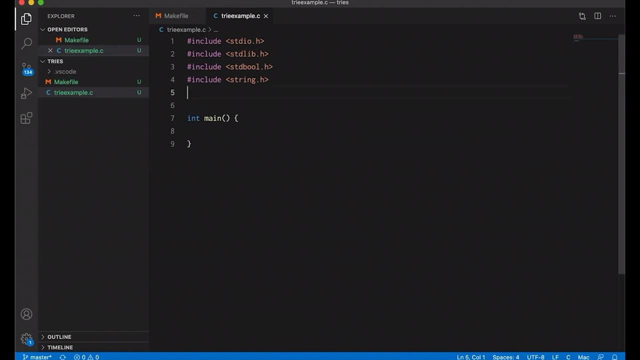 pretty much any other language. Now, let's just start out up here by defining our node. Just like our other tree examples, we're going to have a struct and it's going to let's type def it and it's going to define our node. 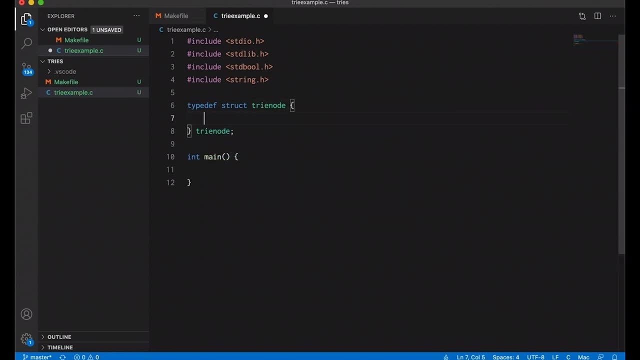 So we're gonna call this try node. okay, Now inside of our struct, one thing that's gonna be a bit different about this node is that I'm actually not going to store the character value of the node in the node, which may seem a little weird. 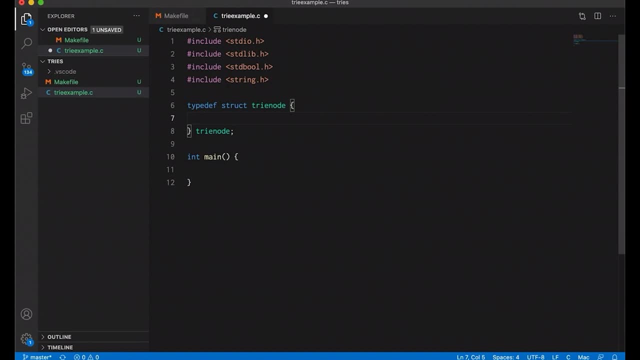 We did that before, before we had an actual value that we stored in the nodes. Today I'm not going to do that and I could do it, but, as you're gonna see, I don't really need to because it's going to be implied. 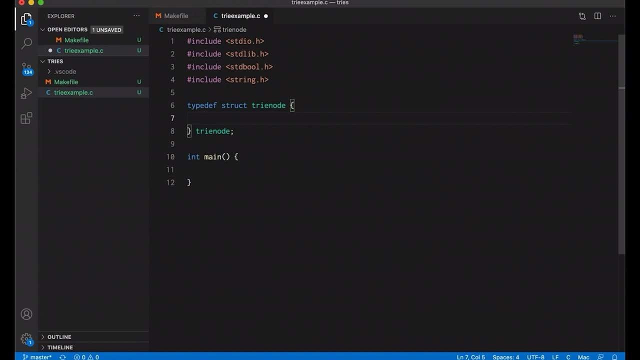 by the links from the parent. So first of all, I'm gonna add a Boolean value here and this is going to. we're gonna call this terminal. This is gonna mark the node to see whether or not this node is the end of a word. 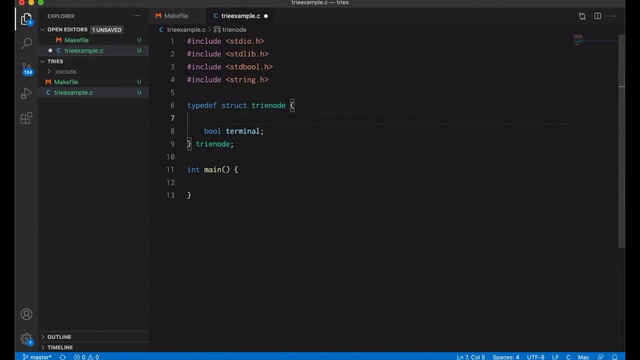 So when I say terminal, all that means is that it's the terminal node of a particular string. And now let's look at adding the children. So we need child links for all the different things that could come after, and our children are going to be an array. 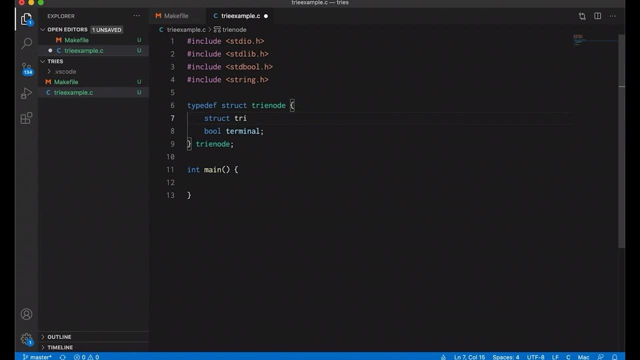 of try node pointers. So I'm gonna do here try node and we'll call it children, And then let's just say we're gonna do the number of different characters in our set of symbols that we wanna consider And each of these pointers is going to tell us: 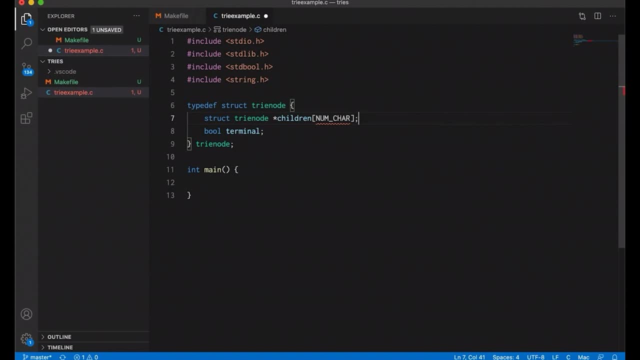 where to find the node for that particular character, And these pointers will also be set to null if there's no child for that character. Now, this array is basically going to be a lookup table. It's gonna act just like a lookup table Again. if you haven't seen anything about lookup tables. 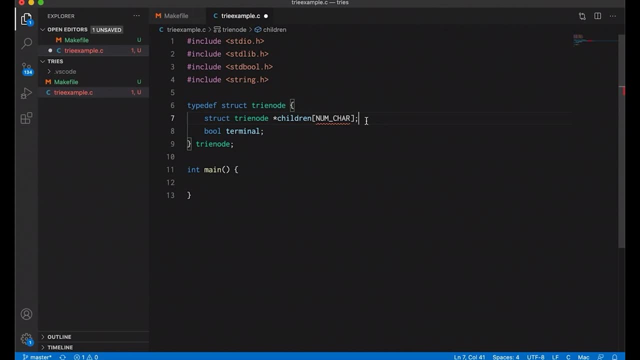 check out my recent video on lookup tables. But note that using a lookup table means that we don't have to search through the list of children to see if a particular letter is there. We just put the value of the character into the array and we instantly know whether or not. 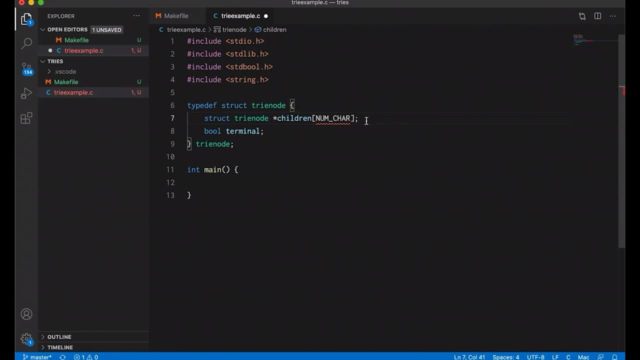 it's a child of this node, And, yes, that does waste a bit of space, but that's pretty common in computer science. We often trade space for speed, and searching for children in this case would be slow, And so we definitely want speed in this case. 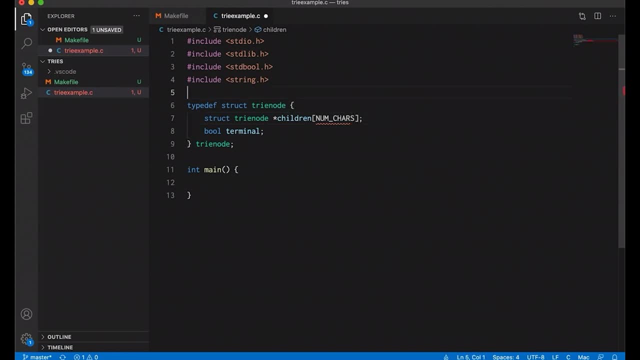 So we do have to decide how big to make this array. For today I'm just going to, let's just set, I'm gonna pound to find numchars to be 256.. And that's because that's how many different values a single byte can have. 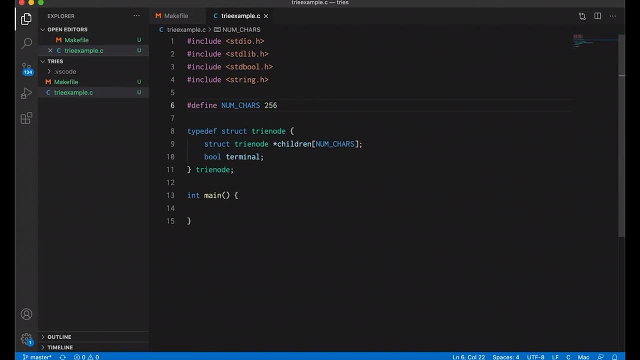 So the upside of that is that basically each of the different characters in my string I will have a next link for I don't have to worry about bounds checking on my lookup table. Of course that is going to waste a bit of space. 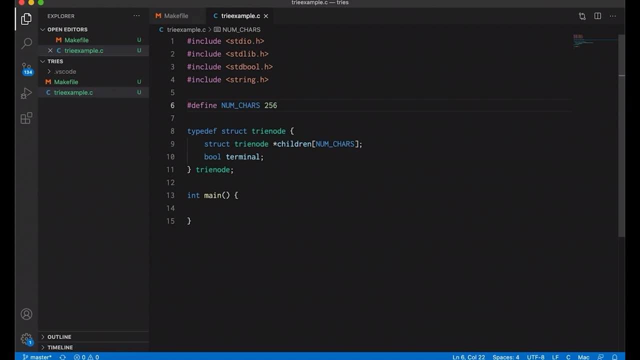 If you wanted to save space and only include the letters or letters and digits that go along with the language that you're trying to support- really whatever symbol set you want- then you could do that And it would give you nodes with fewer children that we use less memory. 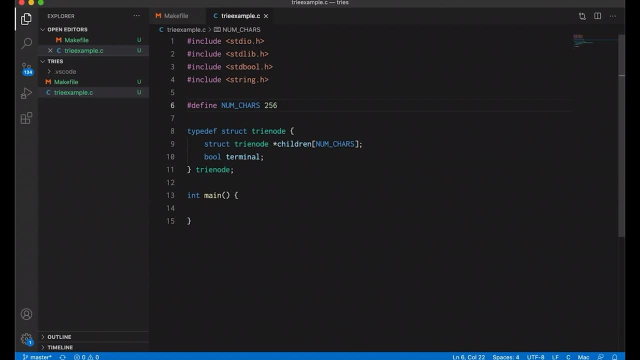 but you would have to do bounds checking, And so for today, I just wanted to be able to store any ASCII string that you throw at me, So I'm gonna use 256.. So this is our node struct. Now let's come down here and start building some operations. 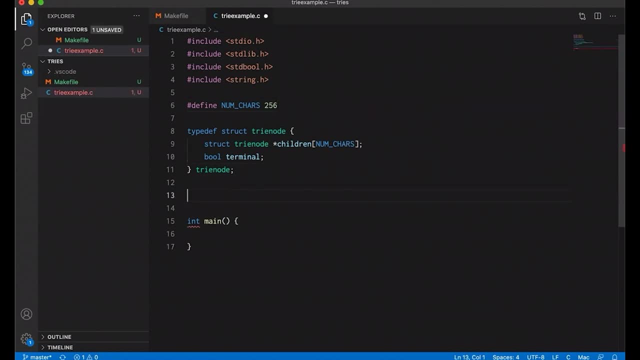 So the first one I wanna make is going to create nodes. I know I'm gonna need that, So let's have it. return a pointer: We'll call it create node. So this is just going to run and it's going to create. 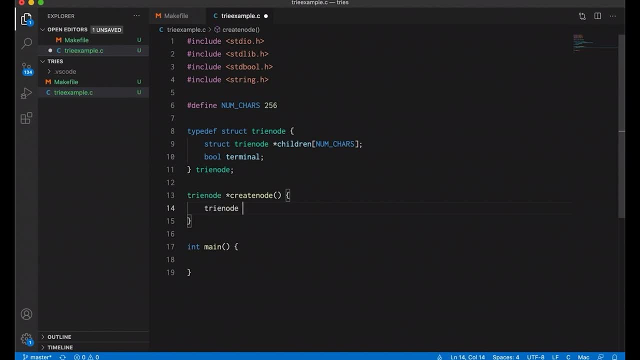 it's gonna allocate a new node and return a pointer to it. So call: make a new pointer, new node and mallet So that'll give us a chunk of memory that can store the new node that we have, that we wanna create. 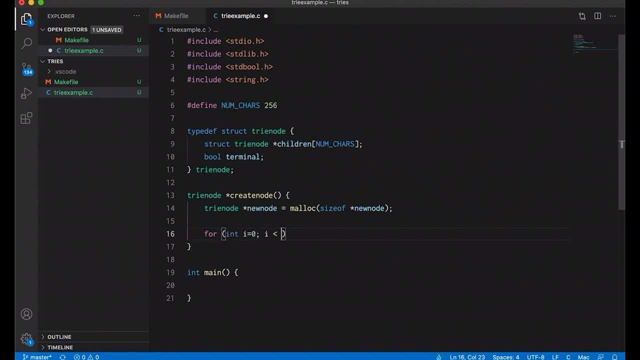 And then let's make a quick for loop that goes through the children, Basically just gonna go through all of our characters and we're gonna set new nodes child. So each of the children, basically the ith child we're going to just set to null. 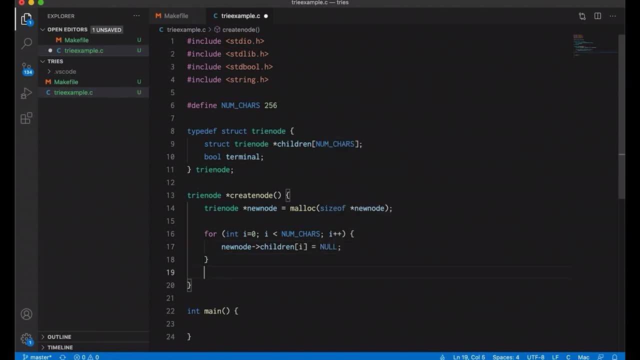 So this is starting out all of our children- links as null, And then we're also going to come in here and set it to be not a terminal, which makes sense, And then we're going to return our new node, So anytime we need a new node. 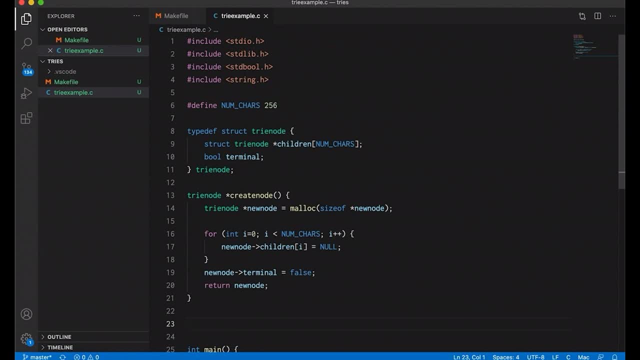 this is going to allocate space for it, And it's going to initialize it to default values, And then we'll change those later on. Okay, so that's what we need: to create a new node. Now let's look at inserting things into our tree. 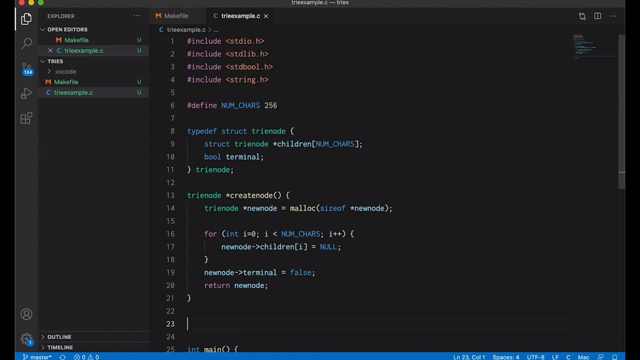 And then we're also gonna print out the tree. Okay, so let's talk about insert. So our insert function is going to return a bool. I'm gonna call it try insert, And the boolean is going to tell us whether or not we actually inserted the new word. 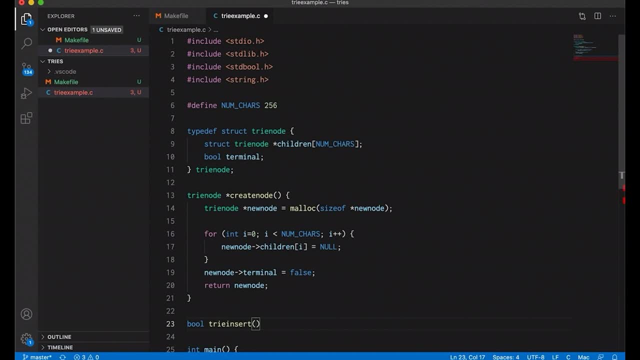 So if it's false, that means the word is already there, The string is already inside our set, And if it returns true, then it means that we actually inserted it And the function is going to take a double pointer. So let's make trino double pointer. 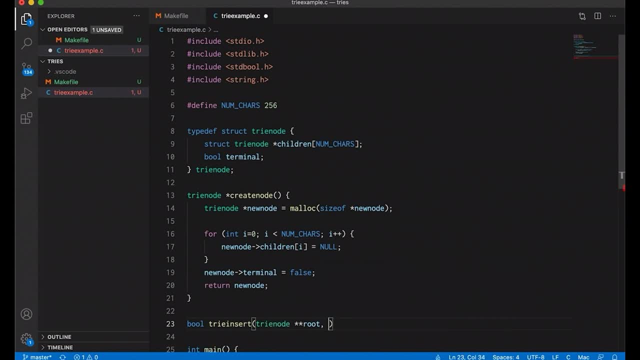 which is a pointer to the root. Now you may wonder why it's a double pointer. I'll get to that in a second. But the second thing I'm gonna add is a character pointer, which is going to be the, the text value that we're trying to insert. 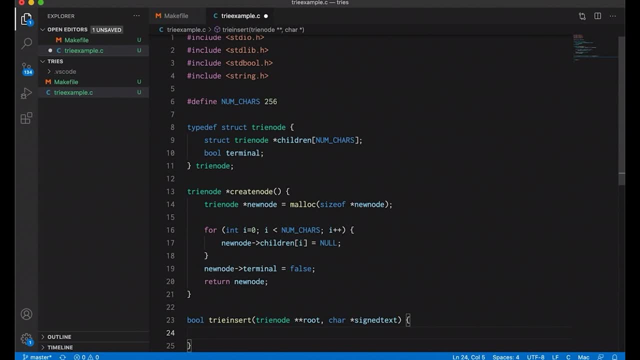 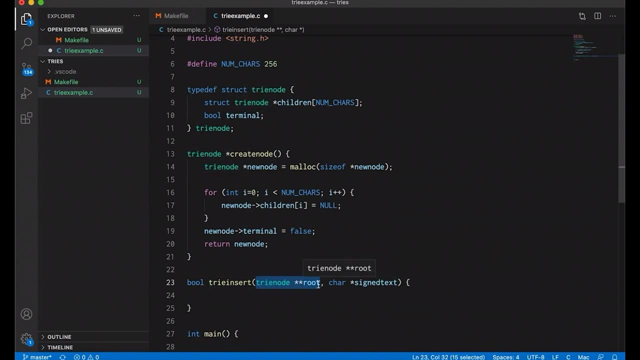 So this is the string we're trying to insert. Okay, so a couple of things that may be a little strange. You may wonder why we're passing in a double pointer here. The reason is is that under certain circumstances, we may want to actually change the root. 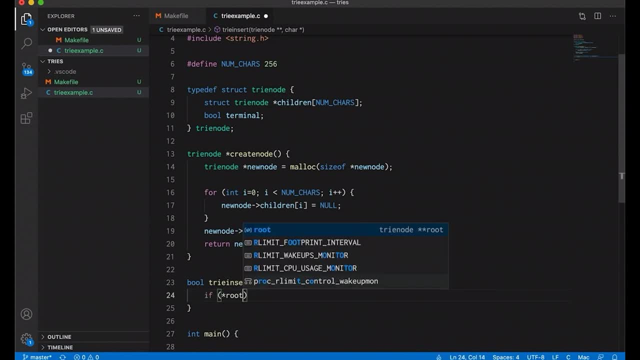 And I'll show you where that actually comes in is like right here. If you say that if the root happens to be null, meaning the tree is empty, then I need to actually set it to a new node, I need to. we're just gonna call our create node like this: 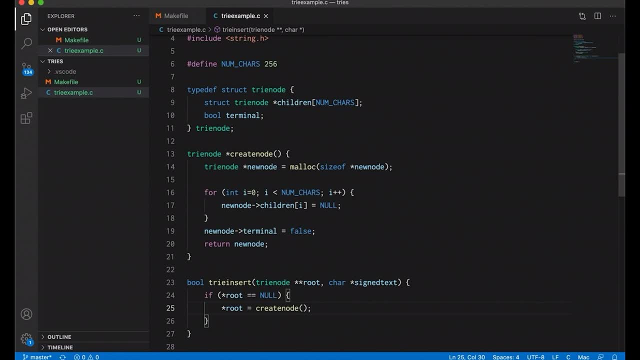 And this is actually going to create a new node and set our root to change the actual root pointer so that it points to that new node. If I pass in a single pointer, that's not going to work because C uses pass by value, And so I'm basically just changing a copy of the root. 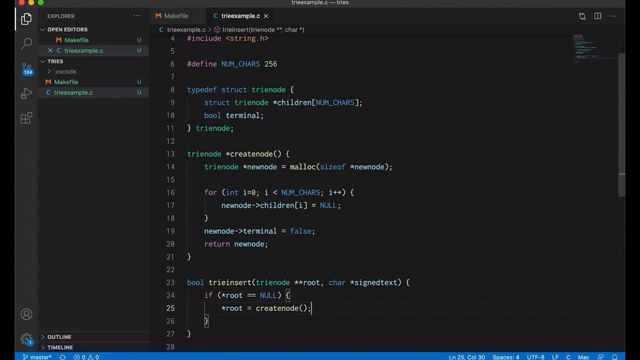 and that's not gonna have the same effect. After this function returns, that change would be null and void. no pun intended. But if we pass in a double pointer, then we can change the value, And so that's what I'm doing here. 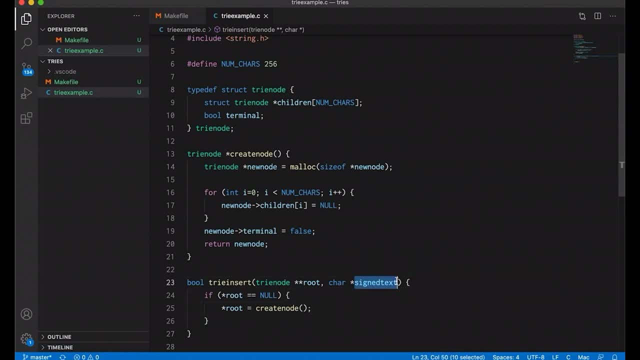 Now you'll also notice something strange: I called this signed text instead of just calling it text. Now one of the challenges is, on some machines, char, you know, the character data type is signed, meaning that it can be negative and positive. 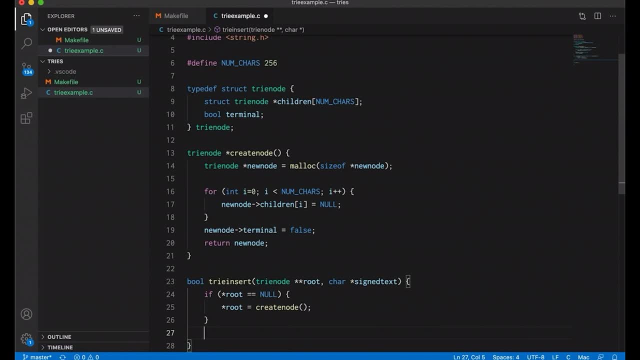 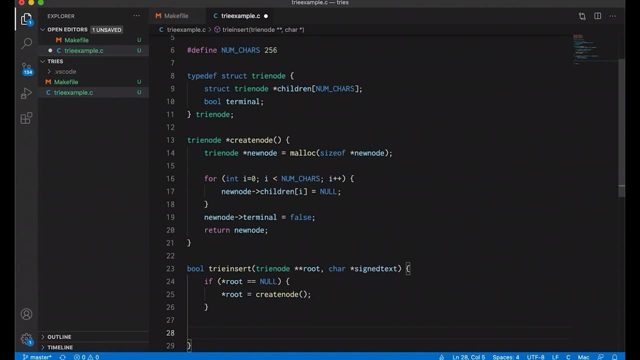 And I really don't want any negative indexes coming into my lookup table. So I'm passing it in as signed, because that's just the normal way that it's gonna be passed in. But I wanna come in here and have an unsigned character. call it text. 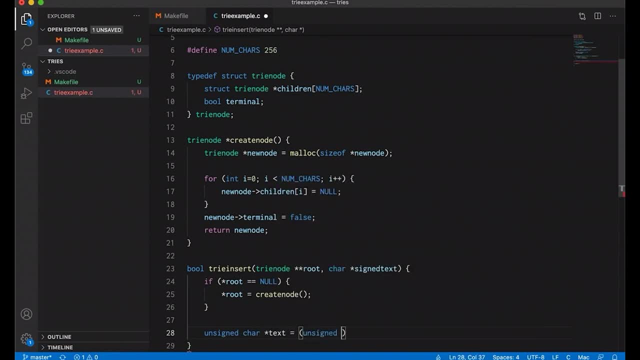 And it's just going to, we're just going to- to cast our signed text to be our text value And then this is what we're gonna actually use internally And this just basically forces all these characters. you know, same number of bits. 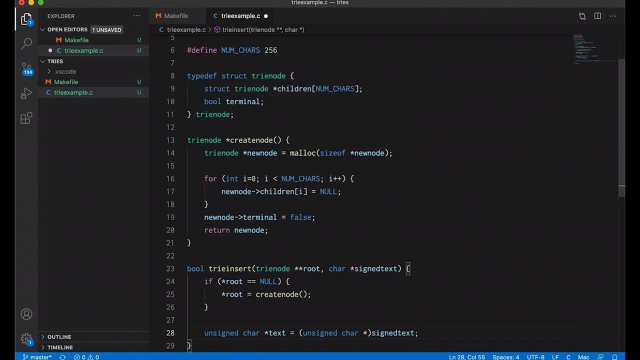 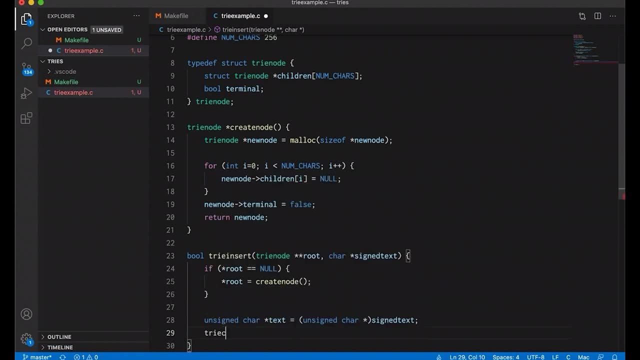 but we're forcing them to be unsigned rather than signed, And that just prevents us from having issues on some machines where we end up getting negative indexes into our lookup table. So also up here I'm going to create a temporary variable. It's gonna be a temporary pointer to a node. 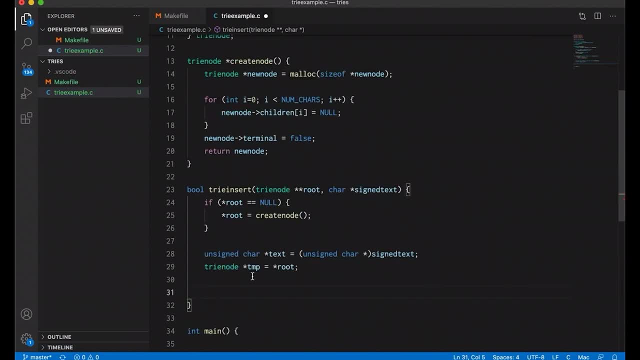 and I'm gonna point it to the root to begin with. okay, So I'm gonna use this for traversing my tree, and it's going to start at the root. That's why I'm setting it to the root- And then we're gonna use that to go down through the tree. 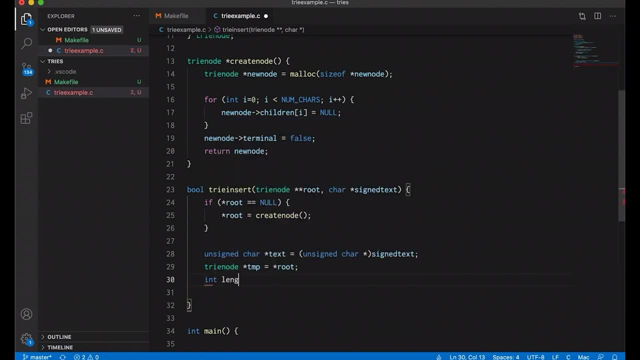 Also one more variable. let's create a length variable, And this is going to be the length of our signed text. So this basically just tells us how far we need to go. So at this point we just need to make a for loop. 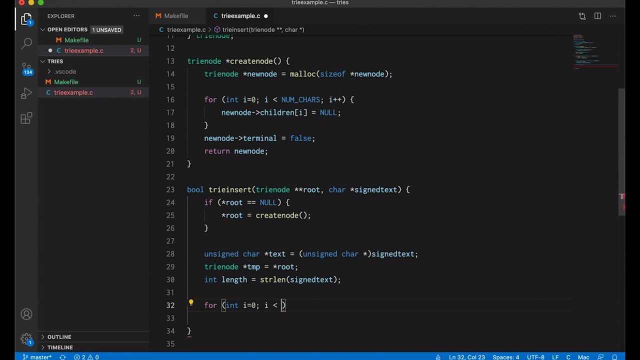 Okay, we know how far we need to go, So a for loop is gonna fit. We basically know how long our string is, And so we're gonna go. I'm gonna take i starting at zero. We're gonna go the length of the string. 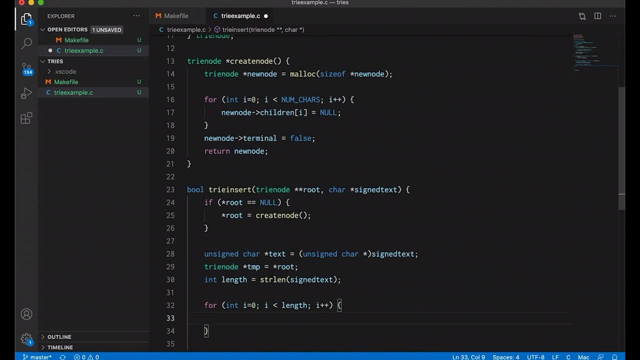 And then each time through here what we're gonna do. we gotta check a few things, okay? So we're inserting so anytime we come in here and we notice that the children look at the child based on the symbol that we see in our string. okay, 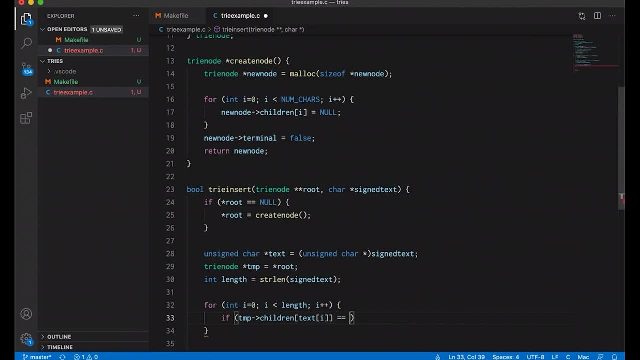 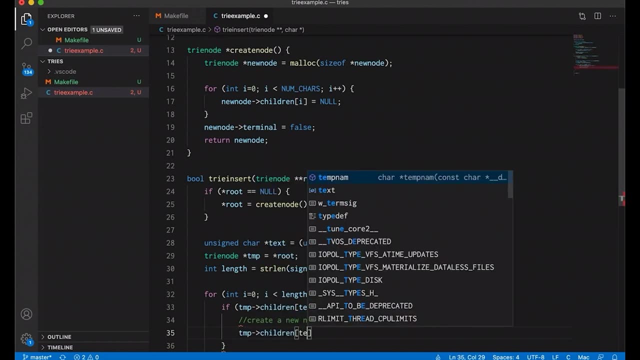 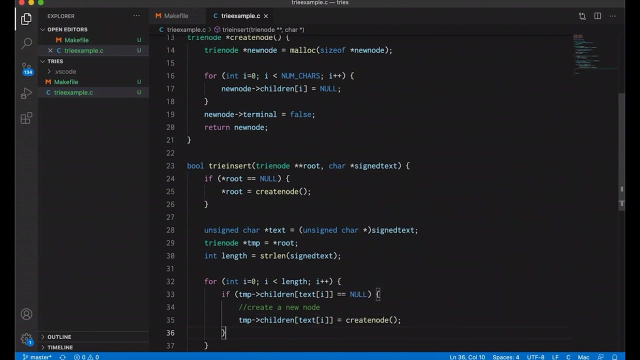 So if this symbol, if the child for this symbol, is null, then simply what we're gonna do in here is create a new node. okay, Children text sub i equals create node using that function we made before And this basically, will just create a new node. 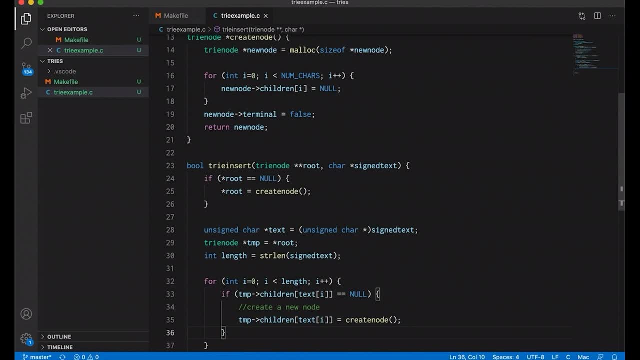 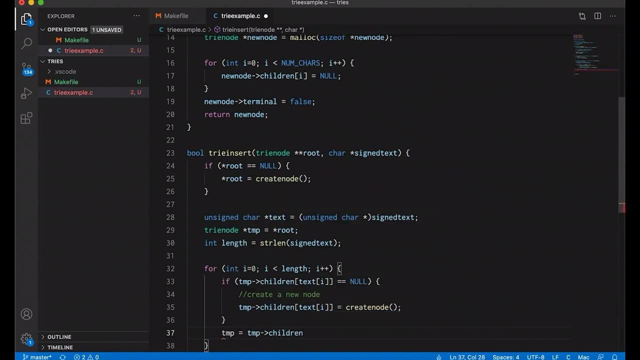 for this child. Now, if it's not null, then we didn't need to create this new child at all And we can just set temp equals temp children. text sub i. So we're basically just moving temp to its child. So we're basically moving through the string. 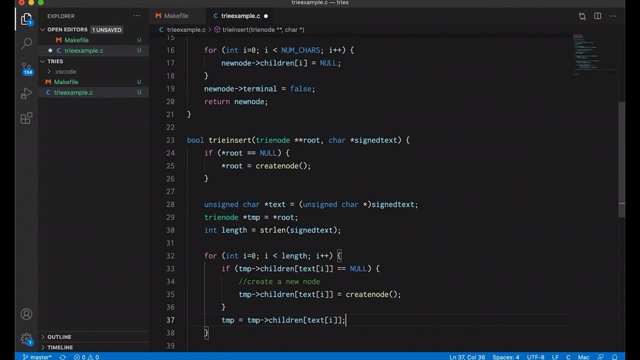 And as we move through we move our temporary pointer to point to the appropriate child child. So we look at the character that tells us where which child pointer we need to look at. Then we look up that child pointer and we follow the pointer down to the next node, And so this: 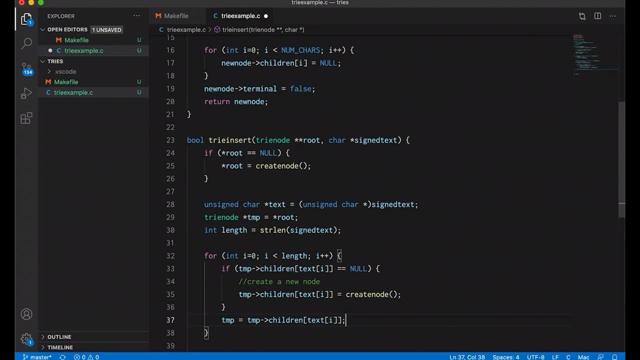 just is traversing the tree according to the characters that were in the string, And if we ever run into null pointers, then we create new nodes for those and fill out that part of the tree. So at this point, once we're done with the for loop, we know we have all the nodes we need. 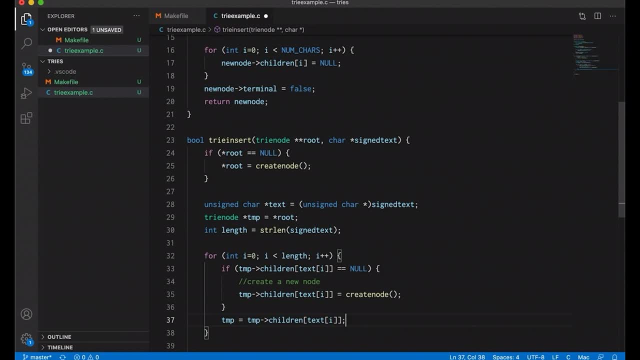 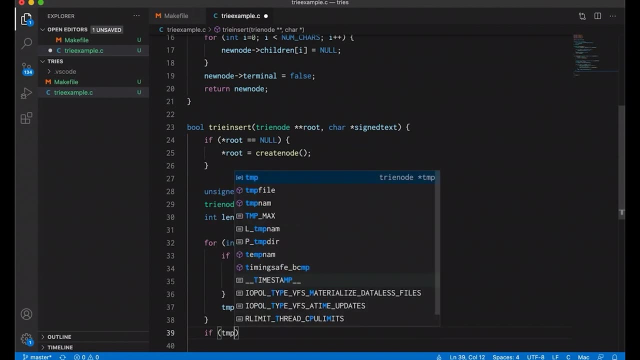 Okay, So now we have to basically try to figure out whether this word is already in the try, And we can do that simply by checking the terminal value of the node. So if temp terminal, so in this case we just return false meaning that yeah, it's already here. Otherwise, 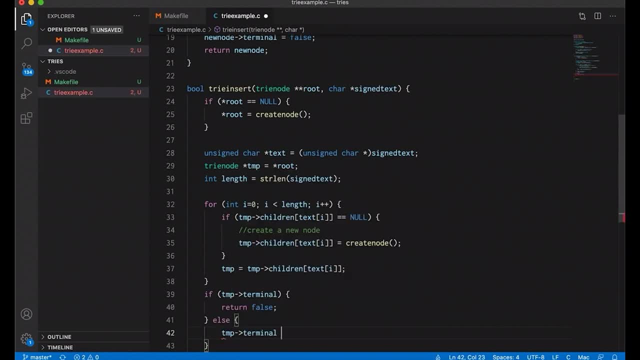 then what we're going to do is set the terminal value to be true, because so it wasn't meaning, meaning that we had a node for this word already in our try, but it wasn't a terminal. So that's that string wasn't actually in the try, even though it had all the nodes it needed, And so 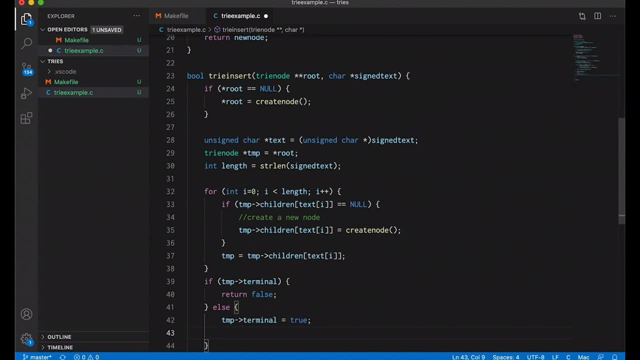 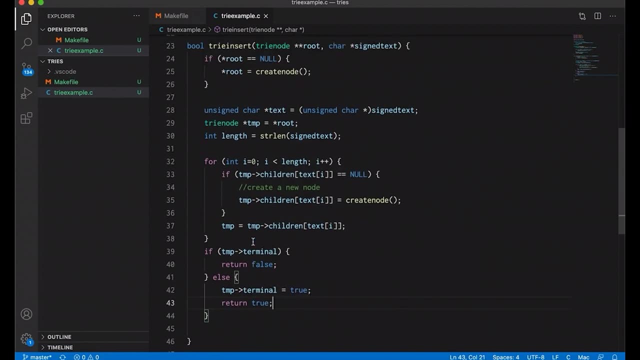 we're going to set terminal in That node to be true. Now that tells it. now it actually is in here and we're going to return true, Okay. So that's pretty straightforward And, unless I did something wrong, that is going to. 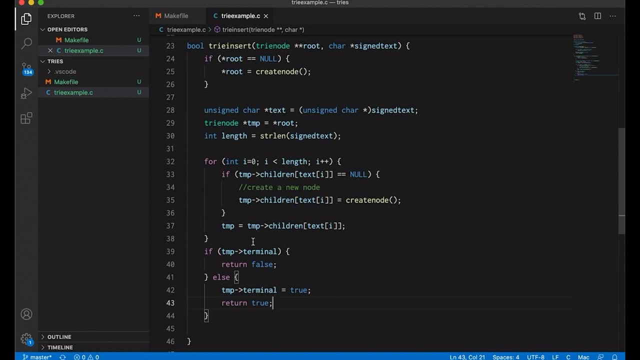 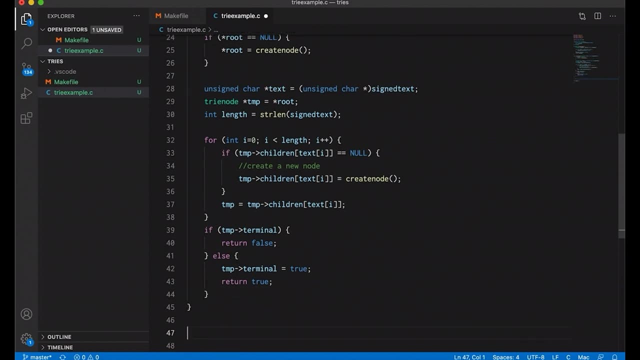 work. That's going to insert a node into our try, So before we test it, we will test it just here in a second. before we test it, though, let's run down here and actually print out our try. I always like to add a printout function pretty early, because it gives me a pretty convenient way. 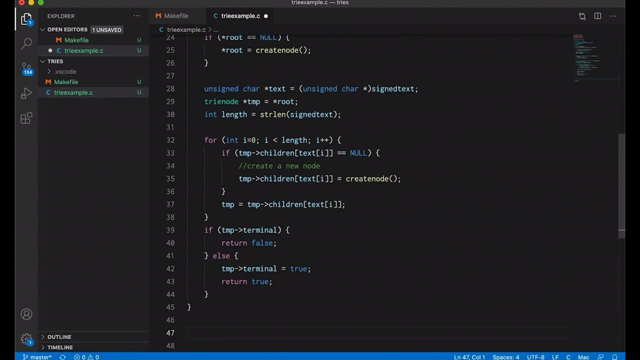 to test out my data structure, just to make sure that the basics are working. So let's make a function called print try. It's not going to return anything because I just want to print it out. We'll pass in a single pointer to the root of our try node, And for this function, 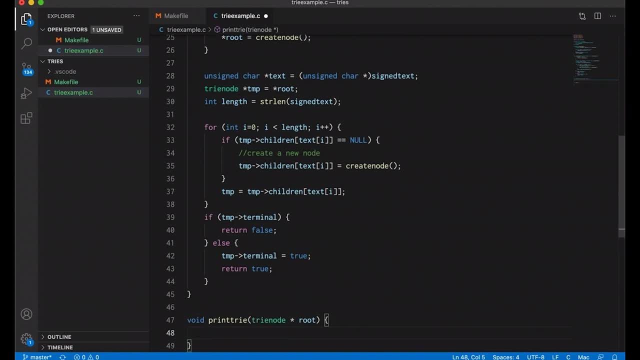 I'm going to use recursion. I've talked about recursion with trees before It just it's so often so nice when working with trees and the try is no exception. So if my root is equal to null- so this is kind of just a special case- We're going to say if it's null, then we're going to. 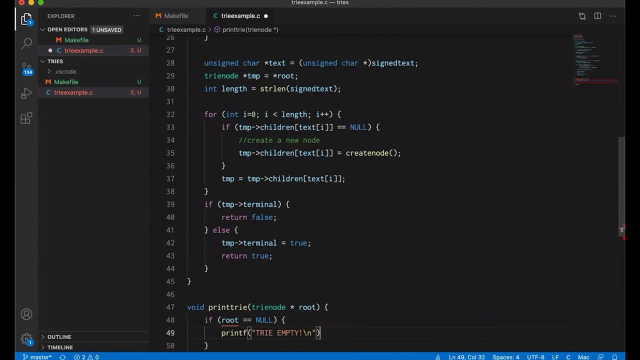 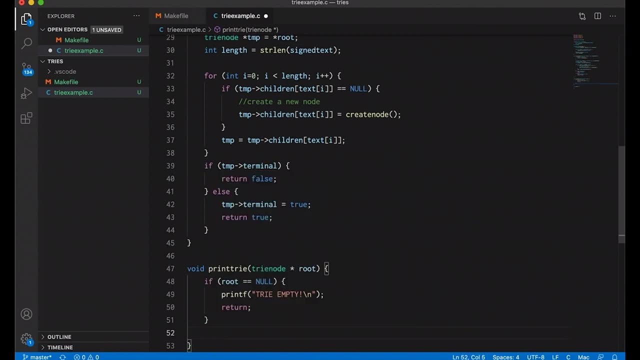 print out try is empty. You can, of course, to whatever you actually want to print out, Oops, And we'll return. So nothing to do here. And if it's not null, then I'm going to go through the children of this particular try. 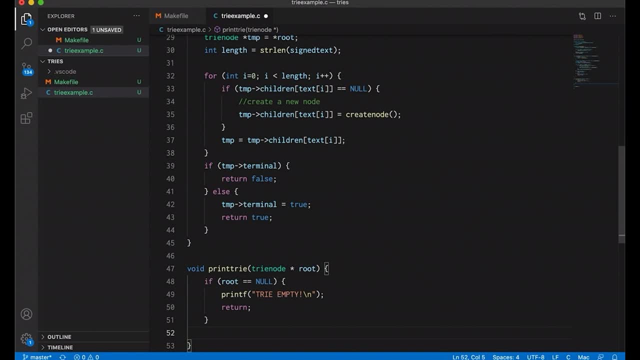 and print out any words we find here. So for this we're going to make a second function. I'm going to call this print, try, rec, because I'm lacking creativity today. So this is going to be the recursive version And I'm going to pass in my root. And right now there are no prefix symbols. 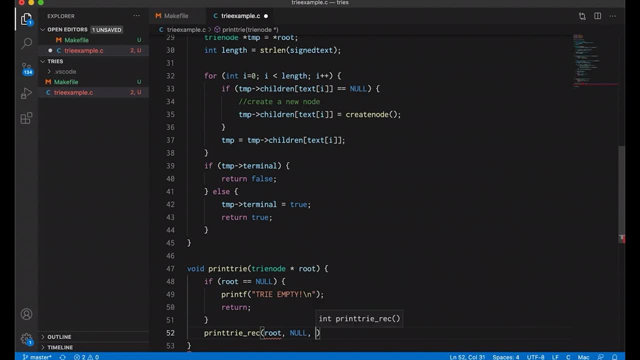 So I'm just going to pass in null- I'll explain this in just a minute- And then the last argument is going to be the number of symbols. So I'm going to pass in null And then I'm going to pass in null- I'll explain this in just a minute- And then the last argument is going to be the number of symbols. 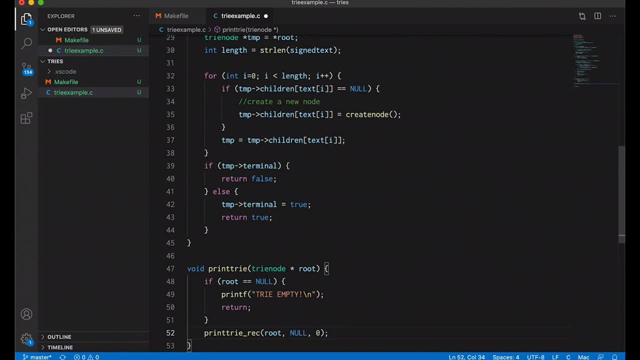 We've seen so far. So that's going to start out as zero. So if this seems a little weird, don't worry about it, I'm about to explain what's going on. So let's come up here and we're going to create this new function, this recursive print, try, rec function And, as you can imagine, 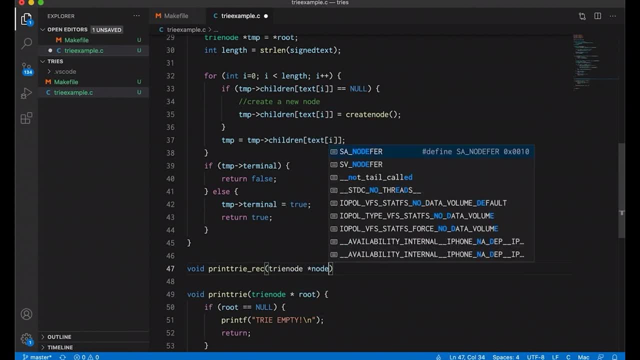 we have a try node. pass that in. That's going to be the current node we're looking at. I'm not going to call it root because it's not always the root. I mean it's the root of a subtree. but I find calling it node is a little bit less confusing to people reading my code. We're going. 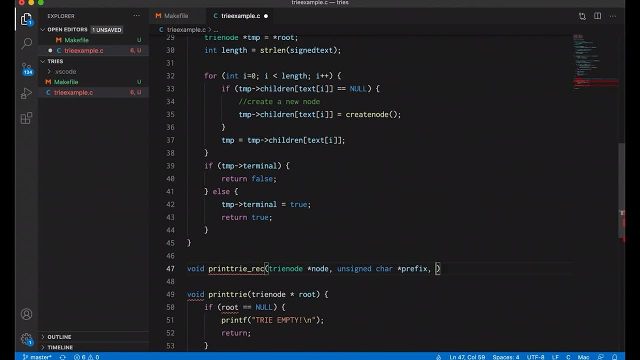 to to pass in a prefix, And this is basically just the history. This is telling us the characters we've seen so far to get to this point in the tree. And then, of course, we also want to pass in a length. Now, I could figure out the length each time, but this is just going to make things. 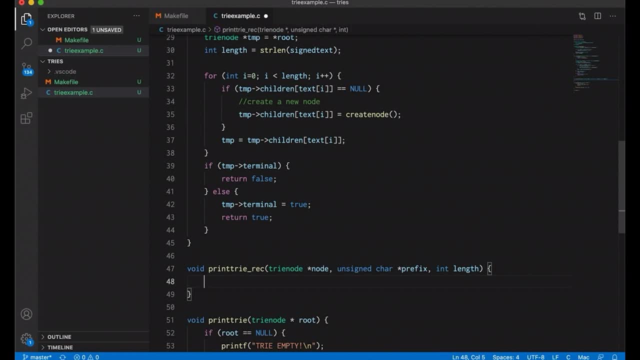 a little more efficient. OK, so now as we get started, we know we're going to need a new prefix when we call down to the next level. So let's make a unsigned character here, new prefix, and it's going to be length plus two. Now, 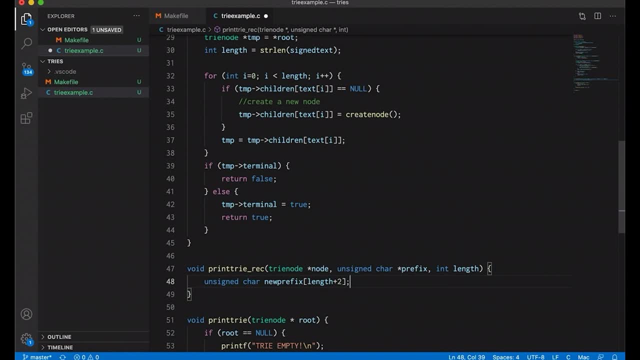 why is it? two is because I need I know how long the previous prefix is and I need space to add one more symbol, one more character And I also need space for the null character. And let's just copy the old prefix over to the new prefix with mem copy And we're going to copy the number of 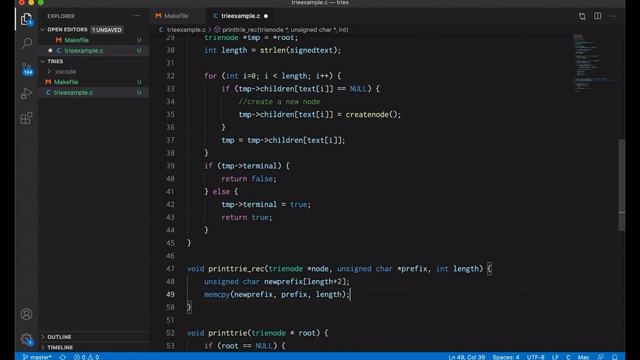 symbols that we had in the length. So this still leaves those last two characters empty. And then, for right now, what I'm going to do is just set new prefix length plus one to be equal to zero. OK, So we're going to null, terminate it. That's important, just to make sure that we don't. 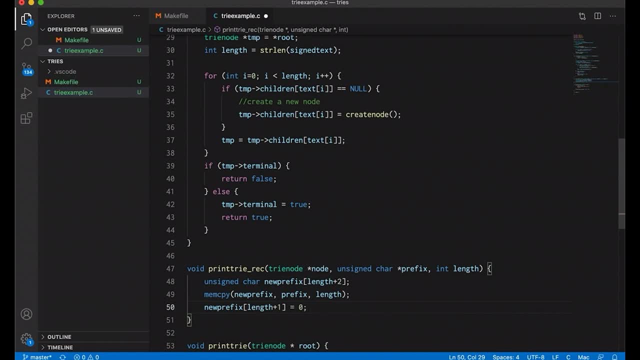 run off into nowhere. Actually, the fact that we're passing lengths around, that's going to be key when it comes time to actually print this stuff out, which we're going to do right here. So our base case is again a recursive function. So you: 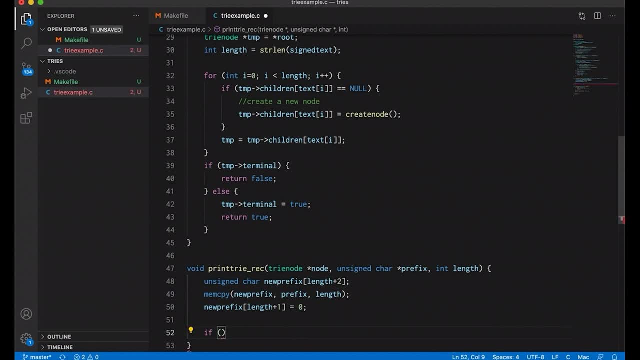 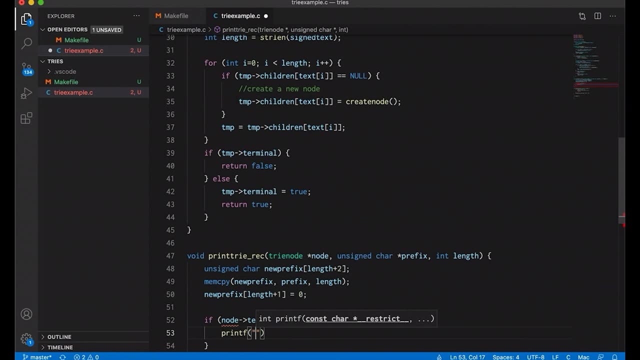 typically deal with your base cases first. Your base case here is going to be: if my node that I'm currently looking at is terminal, then we're just going to print out the word OK, so we're just going to print off. In this case, I'm just going to say word colon and we'll just 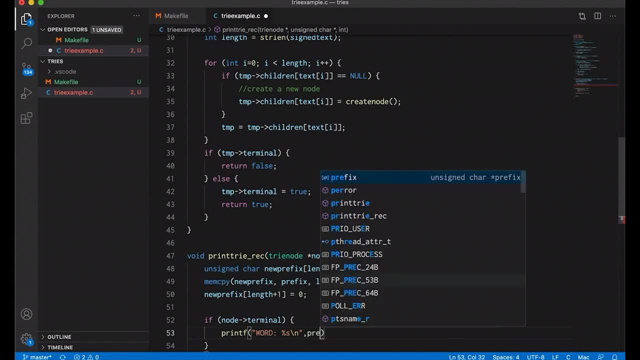 print out the word that we're finding here, And the word is, in this case, going to be the prefix, right? This is the characters it took to get to this point, So we're just going to print out the prefix, And that's great. Now, at this point, we might be tempted to return. We often do at the end. 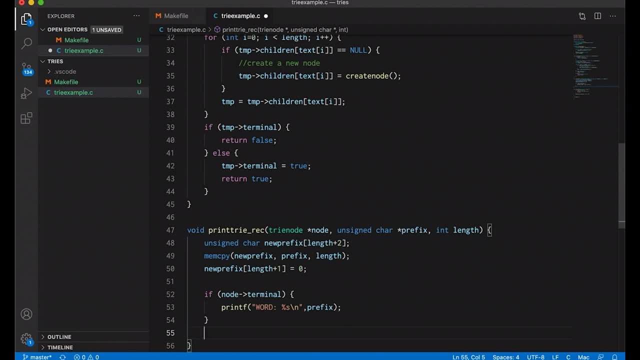 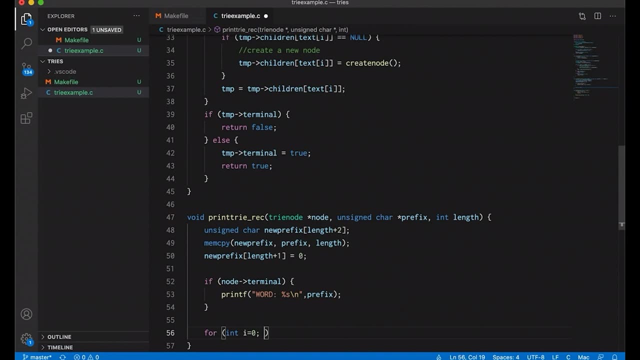 of base cases, but there might be more children below this node, So we actually need to recurse even after we've handled this case. So we'll do this with a simple for loop. Let's go from zero to, in this case, the number of possible children, So the number of characters. 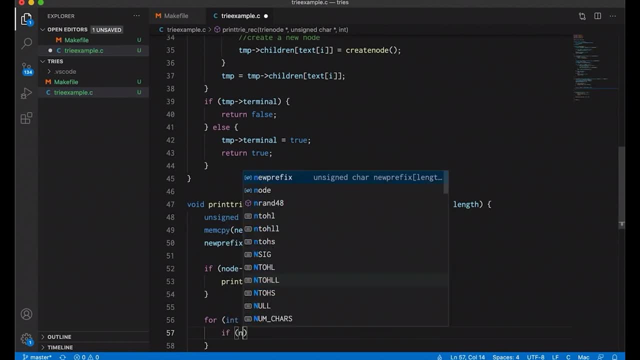 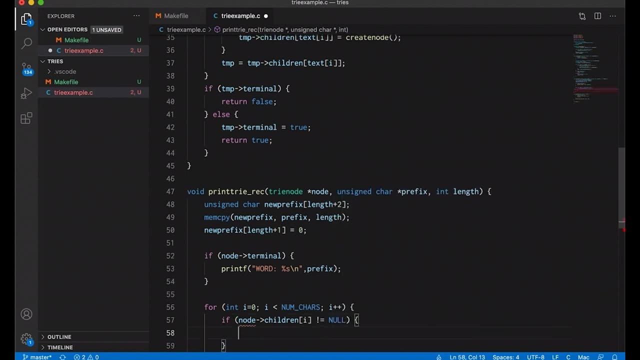 And then we're going to check to see if the child- if it's not equal to null meaning there's actually something down there to look at, because we don't want to recurse unnecessarily. I don't necessarily need this check. I could have moved it as one of the 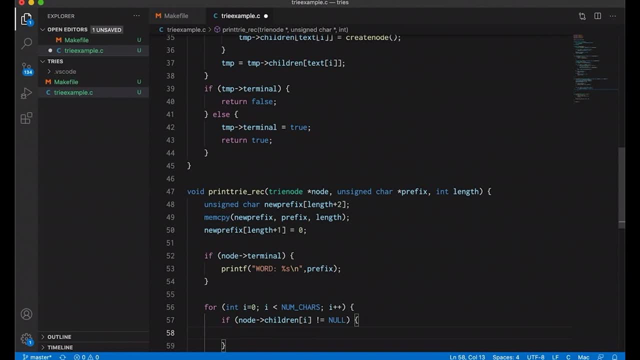 base cases. but that would actually waste a lot of time and a lot of extra function calls And I don't want to do that. So we're going to check it here and then we're going to say: new prefix: length equals I. OK. so this basically is just setting that last symbol, the next symbol in our 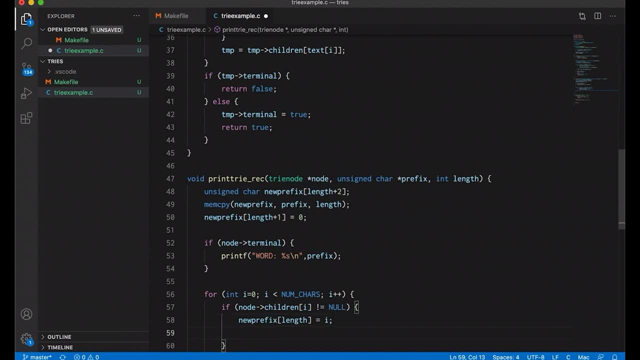 prefix to be the value that we're checking right now, And then we're going to recurse and we're going to call it print, try REC and we're going to call it with the child node this time. So, children, I and we'll pass in the new prefix and we'll pass in length plus one, because we 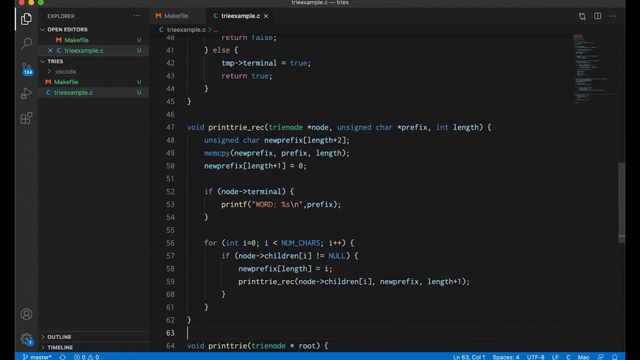 added one symbol to the prefix, And so at this point we're really done. This is going to continue to go through our tree and print out any words it finds, and it will print them out in alphabetical order. Well, let's call it ASCII medical order. 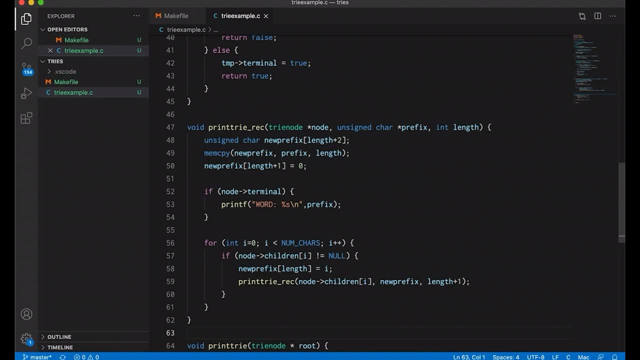 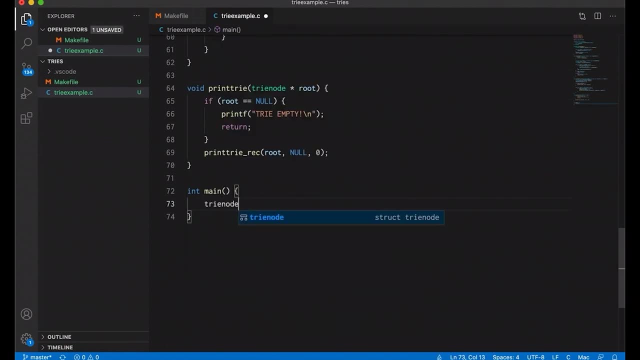 because it's the word that's going to be used for this. So we're going to call it print REC. it's going to just go by the ASCII codes, But this is nice. Now let's come down here and make sure that it actually works, because it's possible that I screwed something up. So let's make a trinode. 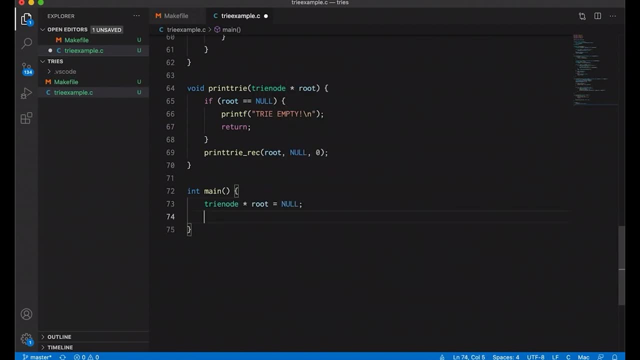 pointer called root, set it equal to null because we're starting out empty. And let's call our try insert function a few times And we'll pass in the address of our root And let's pass in. Yeah, we'll just get a few words. We'll do some of those ones that we saw before, So let's do kit cattle. 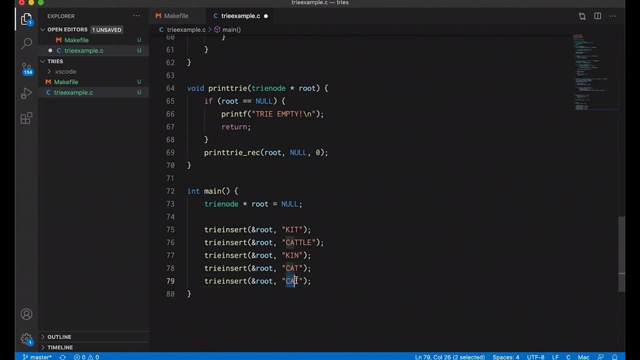 kin cat And let's add one that doesn't fit with these others, Let's do happy And then let's do print, not print f print, try and print, try the root. Okay, great, So this should work, with any luck. I do have a make file over here. Really nothing fancy, It's just like the make files. 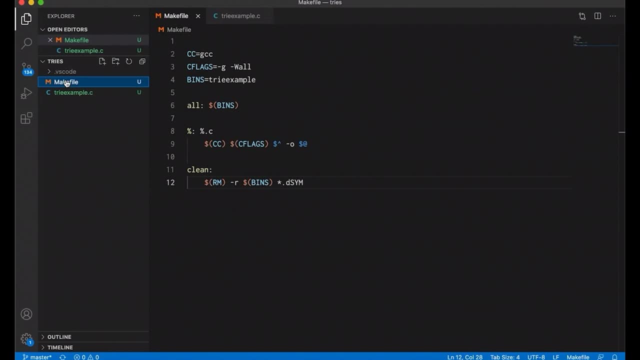 you've seen in all of my other videos. If you've never seen a make file before, please check out my other make videos. They'll give you a quick rundown of how this works, And then I'll see you next time. Bye. 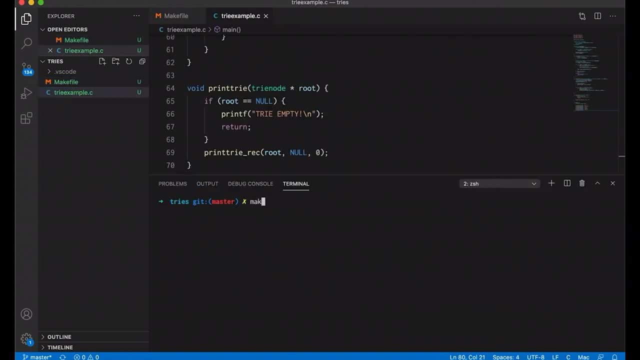 works. But this is going to allow me to come down to my terminal and run make which. let's see, Yes, it did work, Okay, great. And then we're going to run it And you can see, sure enough, it did print. 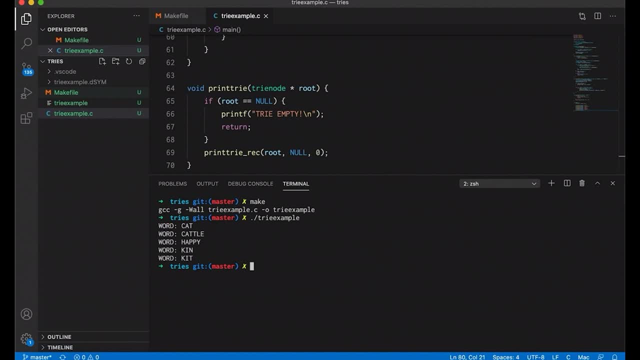 out all of our different strings that we had in the try And it printed them out in alphabetical order. or ask you about a quarter. Now notice, and this is something to keep in mind when you're testing your own code- Notice that I intentionally put these in out of order. The reason I did that. 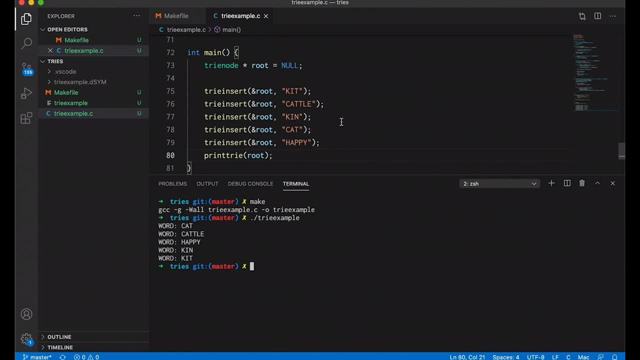 is. I wanted to make sure that the actual ordering was working properly. I want to be able to see that. So that's just something to keep in mind when you are actually testing your code. You do want to make some effort to try to break it. You want to try to give it scenarios where it might. 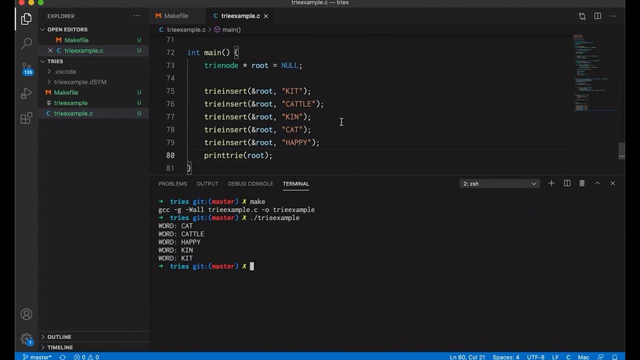 not work. I find new programmers spend a lot of time going way too easy on their own code. They test it without the without really giving it a challenge, And the consequence is that you often don't know whether your code actually works or not. Okay, so now we have the basics of our try. 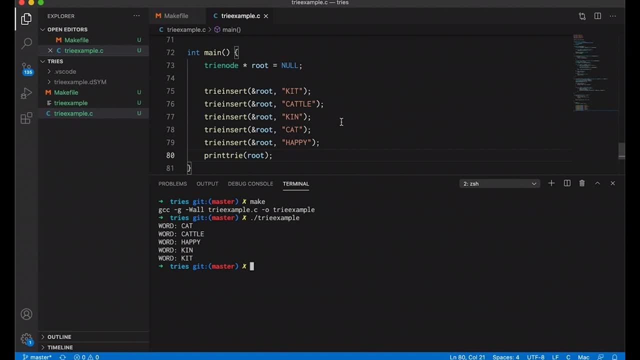 working, And this is where I'm going to need to end for today, just because I'm out of time. At this point we can create and print our try. I know we haven't gotten to searching and deleting nodes yet And we'll get to that in next week's video, And that video will come. 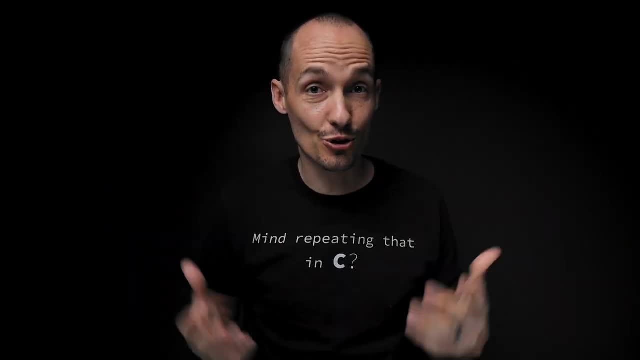 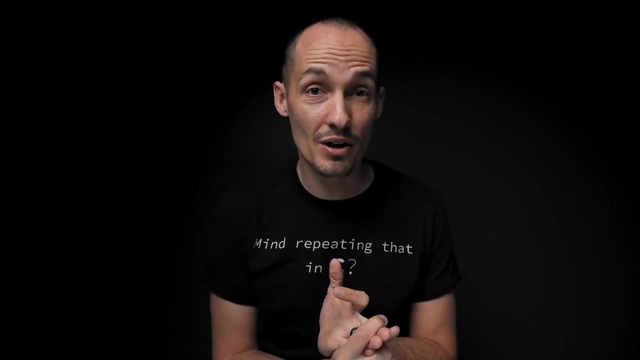 out next Tuesday unless I get some extra time and end up posting it earlier. But I hope this is helpful. I hope it gives you a clearer conceptual idea of what a try is, how it's used and how you could start implementing one. We'll finish this example in next week's video. 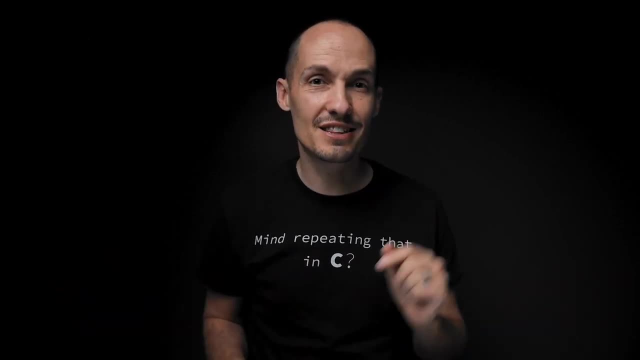 but subscribe to the channel so you don't miss that video and other future videos. like the video, if it was helpful And until next time. I'll see you later.